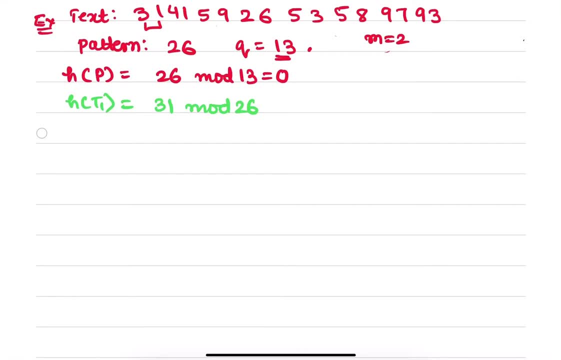 So those who know how to calculate mod or like I, give a scientific calculator method that is a minus a divided by b into b. That is, you go to your pacing method there and just write a mod. b can be written There as a minus a, divided by b into b. 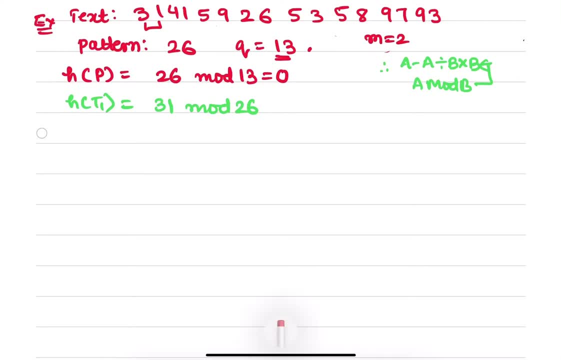 So you can solve that. So, or either this is the like, that's not a huge number, So we can solve by this table of 13.. So it is 13,, 26,, 39,, 52,, 65,, 78,, 91,, 10, right. 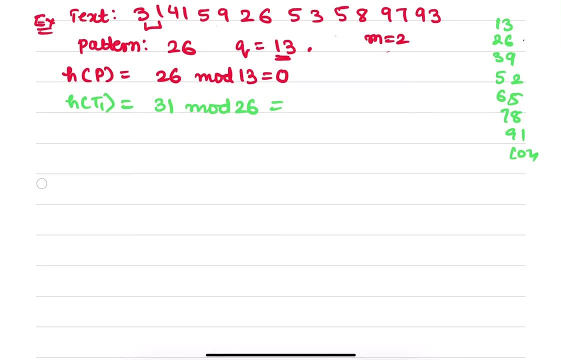 So what is 31 mod 26?? If you see here it is how much 5, right, 26, right, Then hash value of t2.. So what's the second 2?? So that is 14 mod 26.. 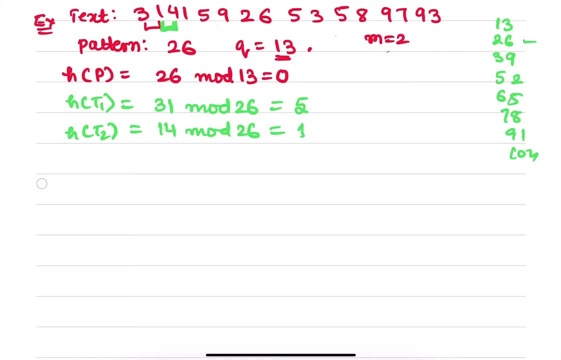 How much? 14 mod 26 is how much It's your fun. So pattern value doesn't matches with the text. Therefore we'll move to the next iteration. Hash value of t3 is equals to 41.. 41 mod 26.. 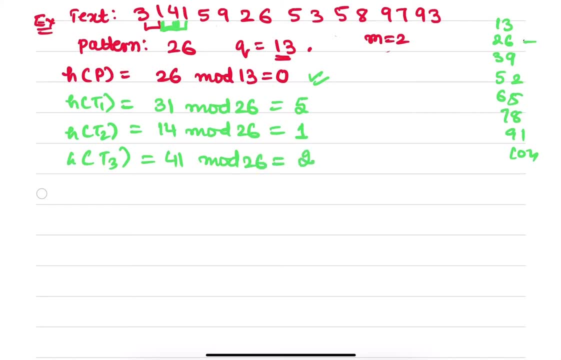 How much it is? 41 mod 26.. That is your 2. 39. So this doesn't matches with the pattern. We'll move forward. So next consecutive character: 15 mod 26,. which is how much? 2, right. 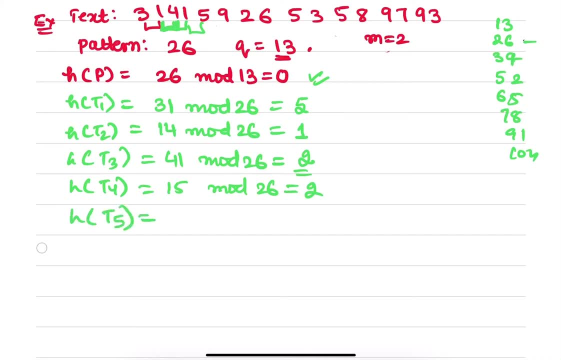 Hash value of t5.. That is your remainder. So 13, 2 is the remainder Hash value of 15 we have take. So next consecutive is 59 mod 26.. So 59, 52 will be there. That is 7.. 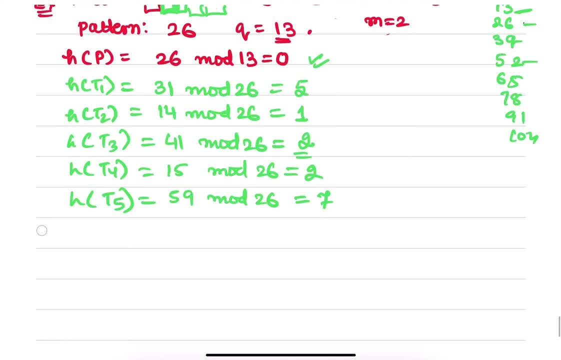 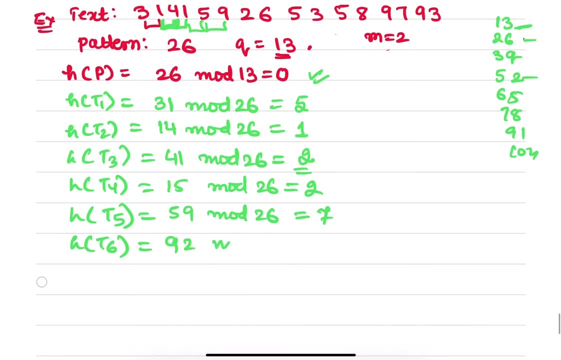 So hash value doesn't matches with the of pattern, doesn't matches with the text subtext: t6, 59 will go to 92 mod 26.. How much 92 mod 26 is 1, right 91 is here. 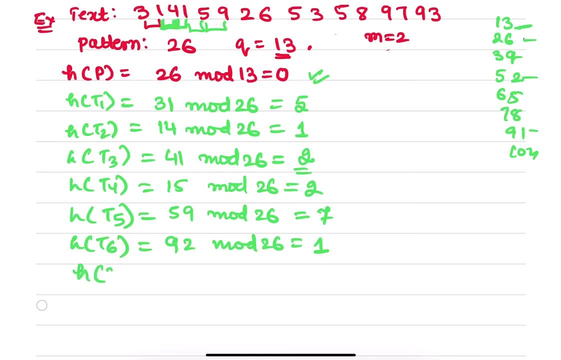 So this doesn't matches. Now hash value of next consecutive is 26.. So 26 mod 26 equals to 0.. Hash value of pattern matches with hash value of t7. Therefore we'll go with the pattern check. So here it is 26.. 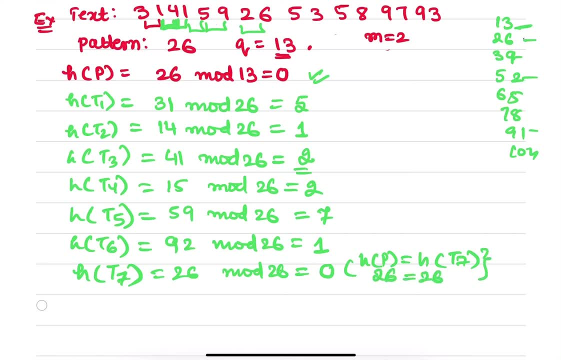 So 26 and 26.. Okay, If I need to find the spurious set, let's say we'll go to the next iteration. So I got this is an actual hit actually. So I got my pattern. but I need to find total number of spurious set. let's say 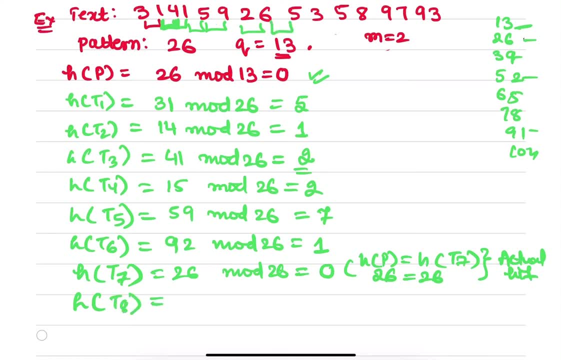 So I will move forward t8.. So what is t8? 65.. 65 mod 26 is how much? 0, right, So your hash value of pattern matches with hash value 8.. But but 65,, oh sorry, 26 doesn't matches with 65. 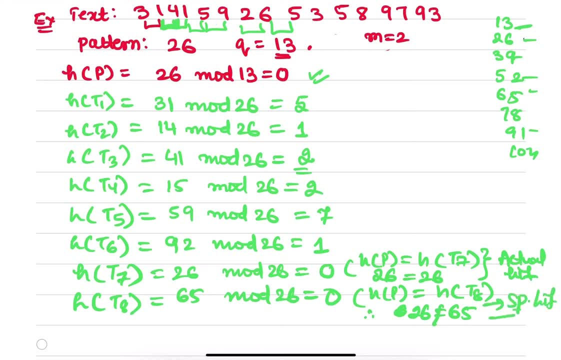 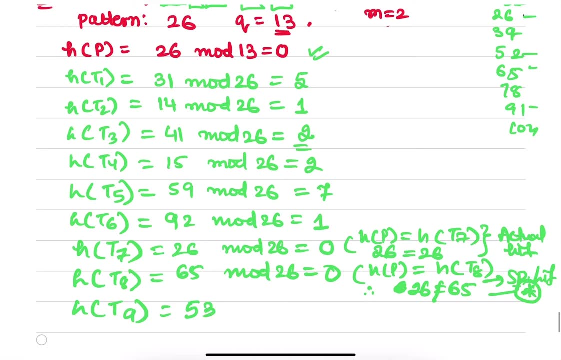 Therefore it's a spurious hit, right. So one spurious hit as of now I have got, Let's move forward. H of t9 is how much? 53, right, This 53. So you have to just solve it. 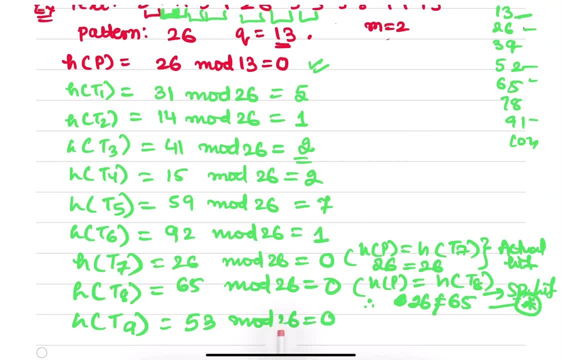 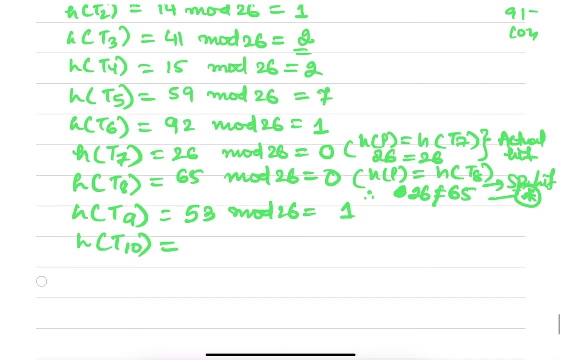 53 mod 26 is how much. Not 0,, it's 1.. 1, right, Then move forward with the hash hash value of t10.. What is it? 53 is done, 35.. Okay, 35 mod 26 is how much. 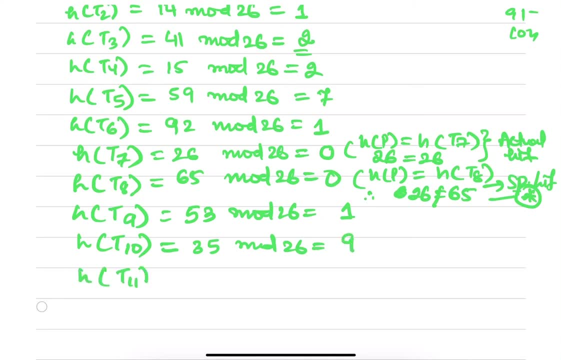 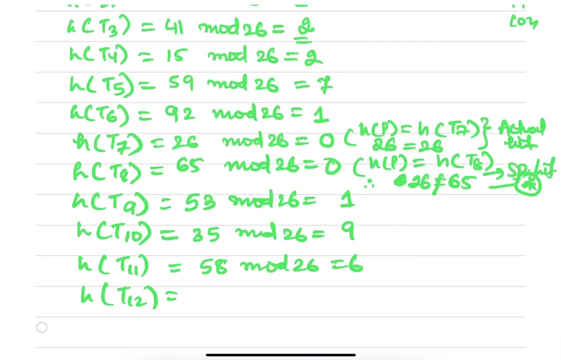 9. So it doesn't matches. t11 is 58 mod 26,, which is 6.. Hash value of t12 is what? 58, 97,, 79,, 93.. So t12 is how much? 89, right. 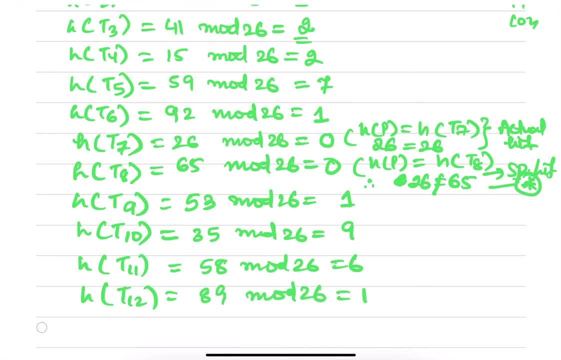 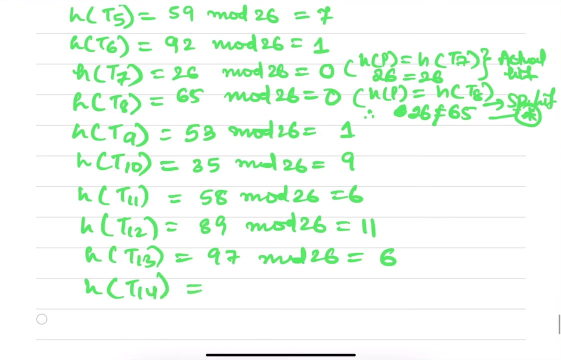 Mod 26 is how much? 11.. Doesn't match Hash value of 13 subtext is 97 mod 26.. It is nothing but 6.. Doesn't match t40,? 79 mod 26 is equals to 1..